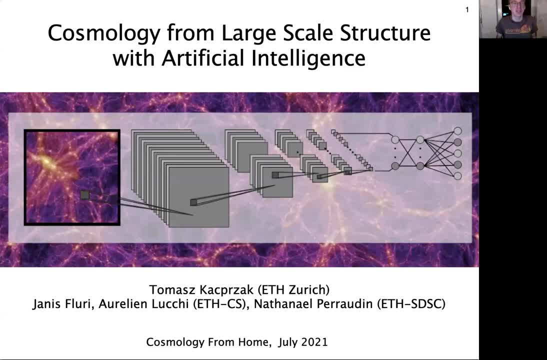 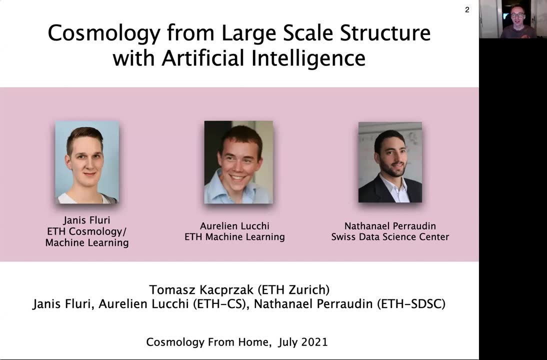 Hello, my name is Tomasz Kacufrzak and I'm at the ETH Zurich. Welcome to my talk about cosmology from large-scale structure with artificial intelligence. Before we start, I would like to quickly introduce our interdisciplinary team of cosmologists and computer scientists. 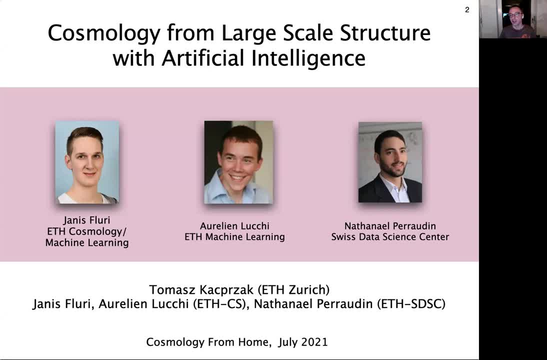 specifically our excellent PhD student Janis Flury, machine learning expert Aurelian Luki and data scientist Nathaniel Paradin. We all work together on these projects I'm going to show today, So let's get right into the topic. Large-scale structure is a powerful 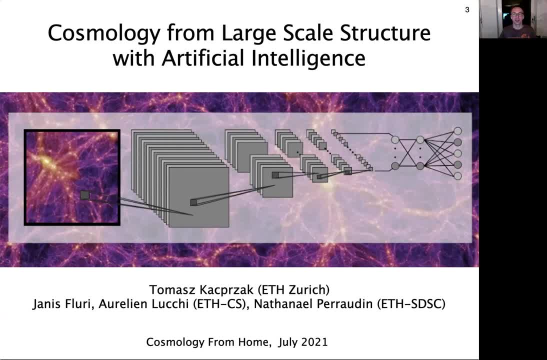 cosmological data set a unique time window into the late-time evolution of the universe. Recently the cosmological parameter measurements started to reach the precision levels comparable to that of the CMB and stage four experiments will provide a treasure trove of data, a great 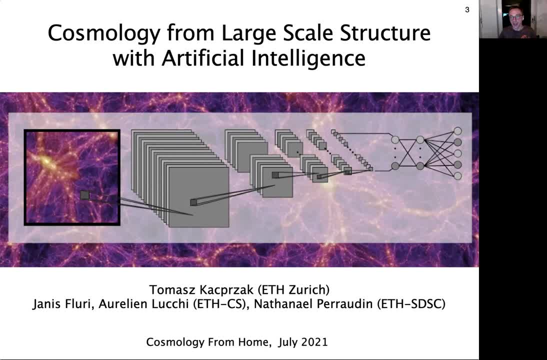 opportunity for discovery, as well as a great analysis challenge. On the other hand, in recent years, artificial intelligence methods have experienced a tremendous growth, providing us with the opportunity to discover new technologies and new technologies. This is a great opportunity to discover new technologies and new technologies. On the other hand, in recent years, artificial 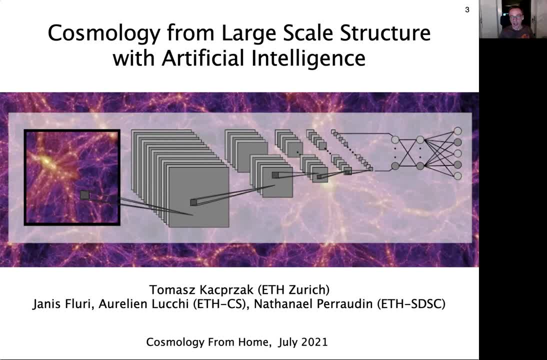 intelligence methods have experienced a tremendous growth, providing us with available and ready tools. In this talk, I would like to show how we can harness the power of artificial intelligence to make more precise parameter measurements from LSS, from the current data, as well as how we can aid and accelerate the analysis of future data sets, So increasing. 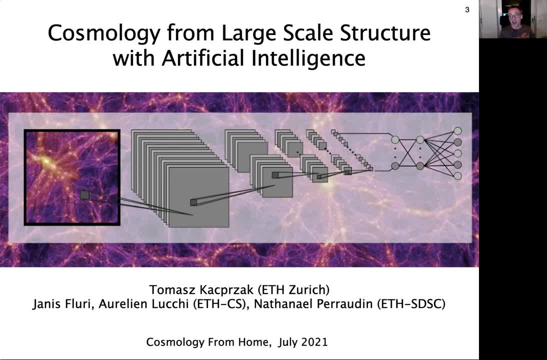 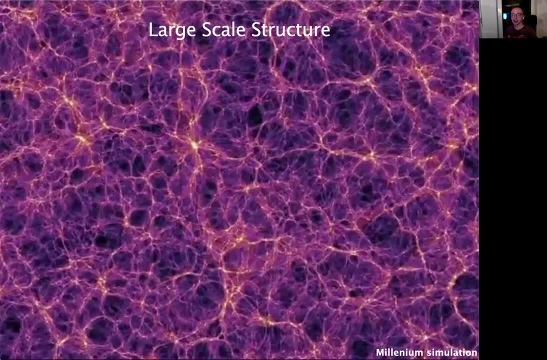 the precision of measurement is what it's all about, especially in the light of recently observed tensions between the late and early universe, for example in the sigma eight parameter between Planck and kids Correct. So cosmological information from LSS comes from pattern structures in the cosmic. 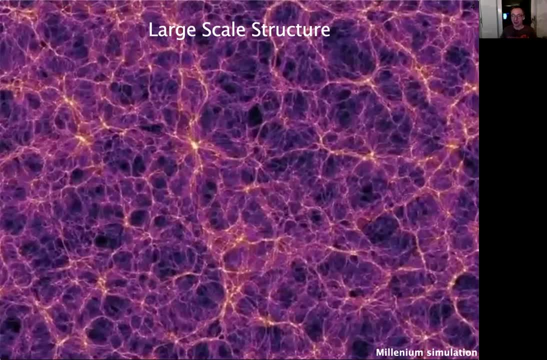 density field In this image. you're probably very familiar with the millennium simulation. you can notice that these patterns are very complex. They create this cosmic web of halos, filaments and voids And also other artificial intelligence methods. draw their, draw their. 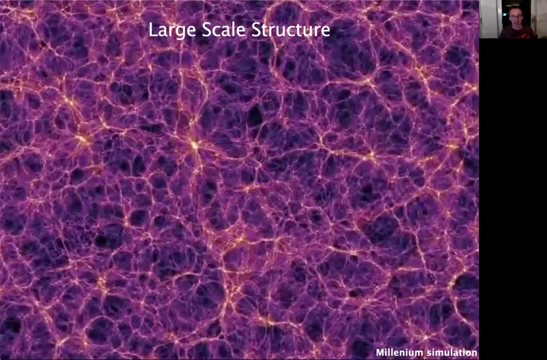 power. power from the ability to construct very complex models, train millions of parameter and capture very complicated patterns in the data. That makes a lot of sense. So let's move on to the next topic, which is artificial intelligence methods such as convolutional neural nets or deep learning, a perfectly suitable tool for modeling and analyzing LSS. 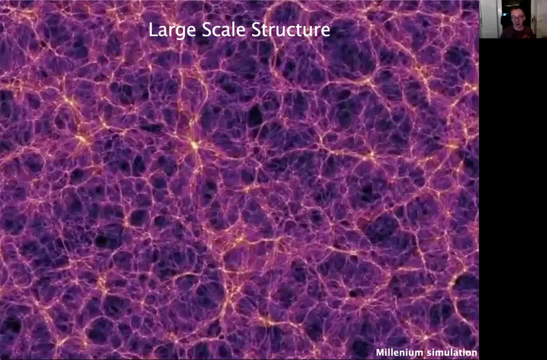 data. So this is where the advantage of AI for LSS comes from: its ability to create these complex nonlinear patterns. So how do we use these tools in practice? Well, we discussed two applications today. First will be to make a cosmological parameter measurements from 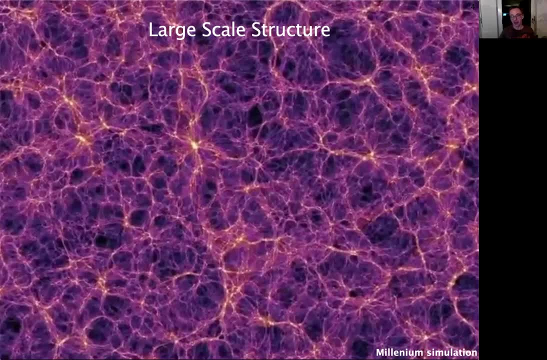 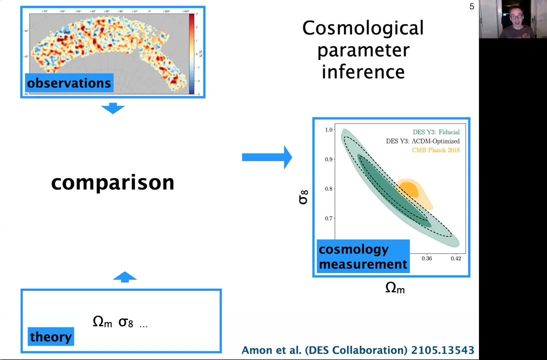 LSS data with AI, And the second is to aid the degeneration of cosmological data. And the second is to aid the degeneration of cosmological data And the third is to aid the degeneration of cosmological simulations using generative machine learning models. So, if you would like to generally measure some parameter constraints, 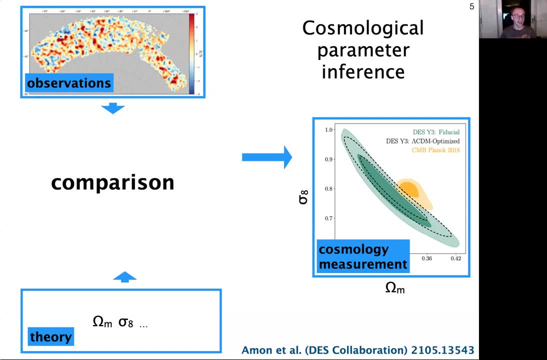 from our large structure data, for example with gravitational mass maps. we have some theory that with parameters we would like to constrain. We use that theory to make some kind of prediction And we compare it to the data And from that we get our cosmology. 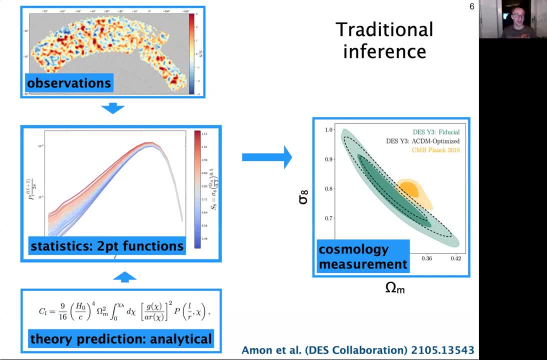 theorem. Traditionally this is done using a chosen summary statistic, for example, most commonly the two-point functions, power spectrum or correlation function, And the theory prediction is then tailored for this summary statistic. So this theory can be analytical or semi-analytical. This one statistic is used for comparison in Bayesian framework. 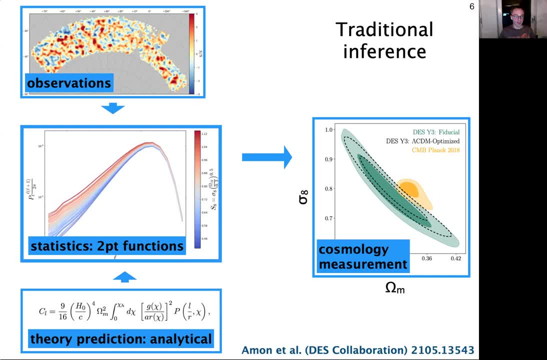 to put constraints and parameters, So the power spectra and all other parameters we use. this formula was given a first step to a better understanding of the model and the computational dynamics of the model And other hand-chosen summary statistics will always only probe a specific part of information. 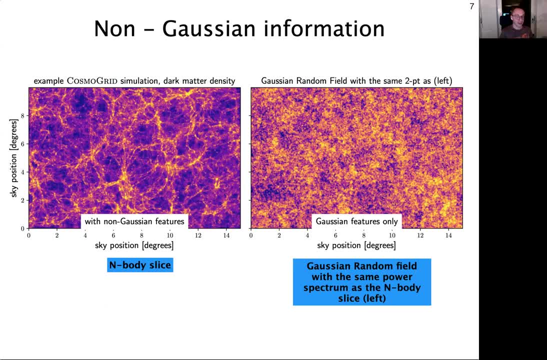 that's contained in the data PowerSpec track will capture only the Gaussian information, And there is, as we saw in the previous millennium simulation image, quite a lot of information that is highly non-Gaussian in the density field. So this is an example of a light cone shell. 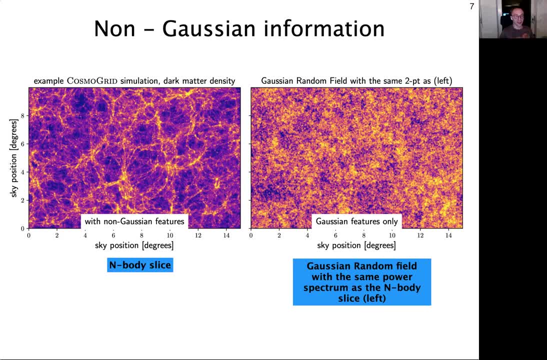 that we use in our cosmological simulations, which on the left from the NBody simulation PKD graph and on the right, this Gaussian random fields draw with the same power spectrum as the image on the left. So you can see that the complexity of patterns. 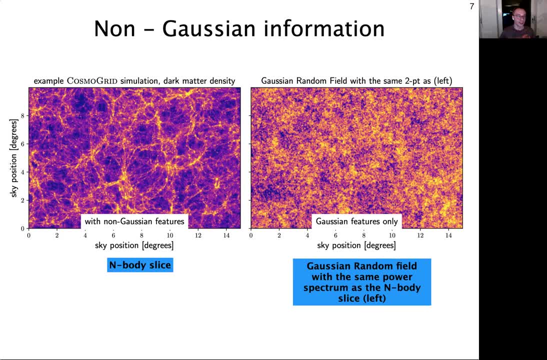 that the Gaussian random field can create is much smaller than the one in the dark matter. density- And this is the part complexity- we want to harness to make more informed parameters, And we're gonna leave that to the measurement Now, in this new inference paradigm. 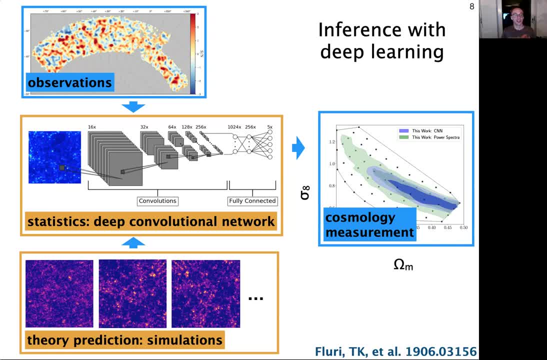 we would like to use a machine learning tools to automatically detect features that are present in the data that will be useful and informative for a cosmology measurement. Instead of choosing a fixed statistic, designing it ourselves from using our intuition, we let the machine find the most informative. 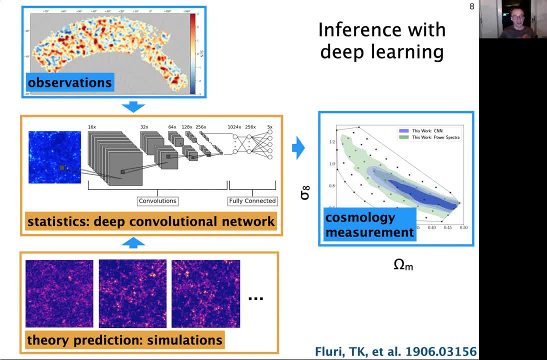 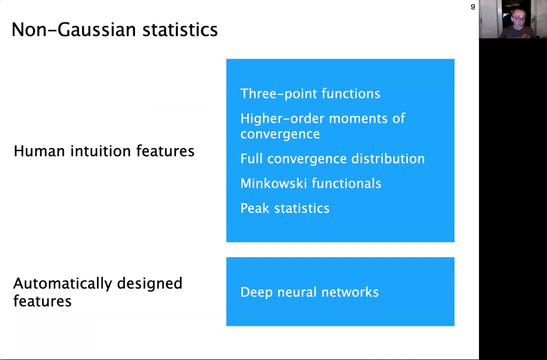 and relevant patterns. This comes, of course as a cost uh the machine with uh uh simulations directly, so we can only do it for a grid of simulations in a smaller parameter set given by our computational cost limitations. so just to note, there were other summary statistics that were designed to probe the 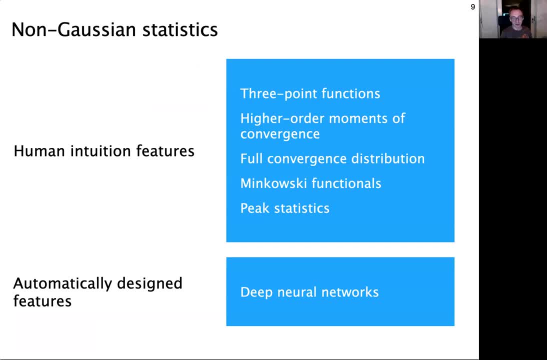 non-gaussian information, for example three-point functions, minkowski functionals and peak statistics. they're all very interesting and um, there's also- i'm working on- some of that kind of analysis too, and but um what fundamentally different? what is fundamentally different about deep convolution? 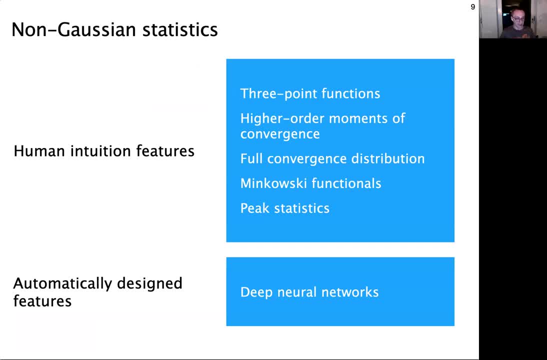 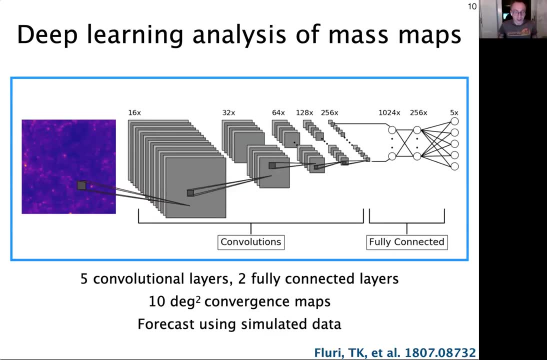 neural nets and ai tools in general is that it uses automatically designed features. so with that potential for improvement coming from ai, we asked ourselves a question: how much exactly will we gain using deep learning analysis? so in this first feasibility study, led by janice, we used the 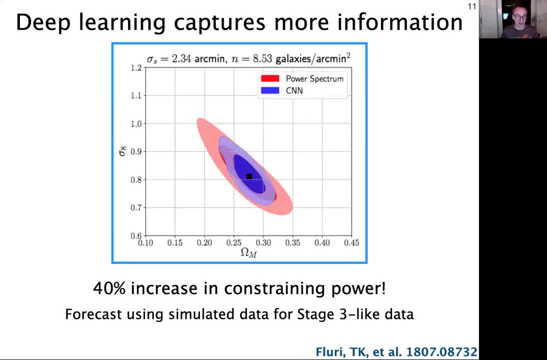 relatively simple neural net and we performed an apples to apples comparison between a power spectrum analysis and a convolutional neural net analysis on a stage three. like survey set up for weak lensing and we noticed that, for a kind of a reasonable assumption about smoothing scales, we gain around a 40 percent increase in the constraining power using convolutional neural. 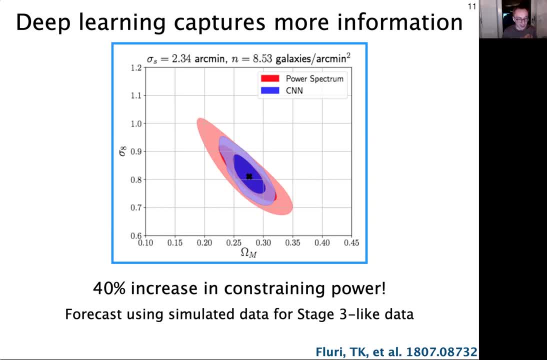 net compared to the power spectra, and this is a very significant gain, given that we would like to reduce the amount of data. so we would need a roughly twice the amount of data to reach the same advantage using power spectrum only. um, so this is very promising. um. we also explored different 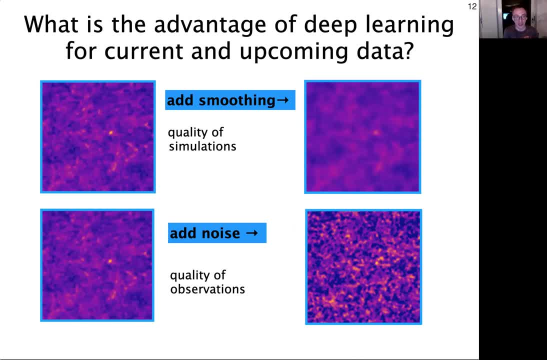 survey configurations and different um quality of theory prediction and that we will be able to use for the deep net and deep learning measurement. so if our um quality of um, our simulations, will dictate our smoothing scale, so of course um our ability to simulate small scales will have a huge impact on how much we can gain. 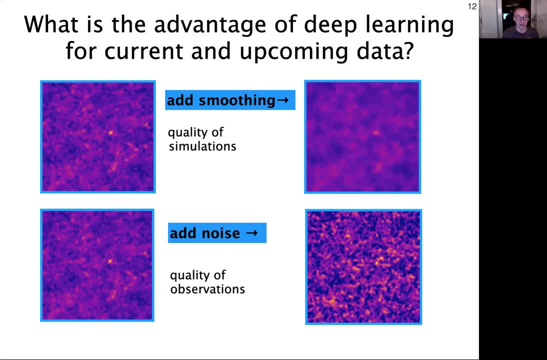 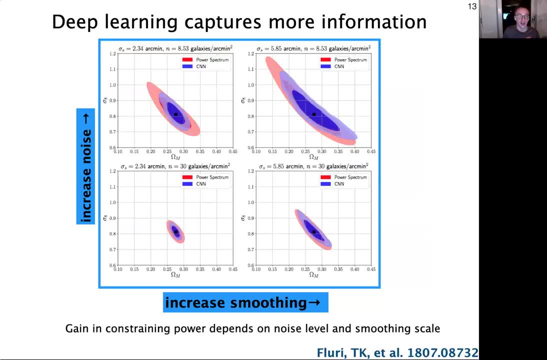 um and, of course, uh, the noise coming from the survey. depth and survey size will also impact the quality of measurement on the observation side. what we found out is that, as we expected, if we include- only if we include- smaller scales in our measurements, so our smoothing scale is low, the deep learning gains. 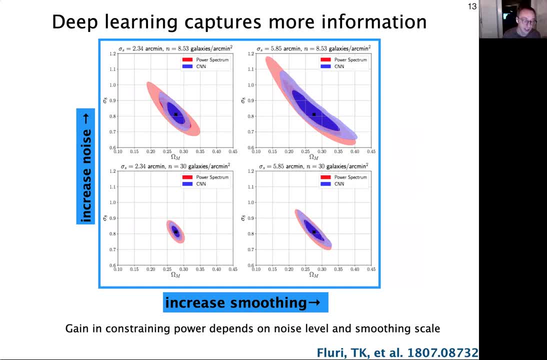 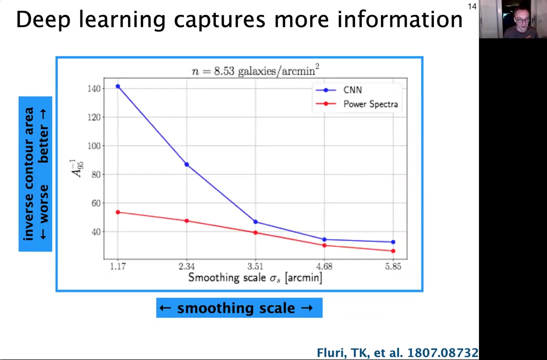 um more. it gives a bigger advantage over power spectrum. if we increase the smoothing scales, we lose the advantage. on the other hand, if we vary the noise level, the results are um consistent: the advantage is maintained. so even for relatively noisy data sets. deep learning captures more information, and this is the previous plot summarized in a on a, on a curve. so on the smoothing. 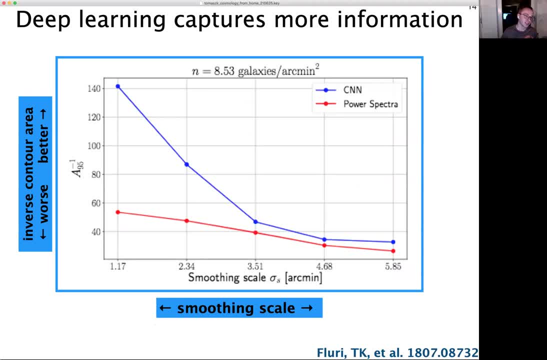 scale is on the x-axis, and the x-axis is on the left and the smoothing scale is on the right. so um advantage of um, um, the deep learning analysis compared to power spectra on the y-axis, so higher is better, and if we go to small smoothing scales, of course CNN's advantage gets. 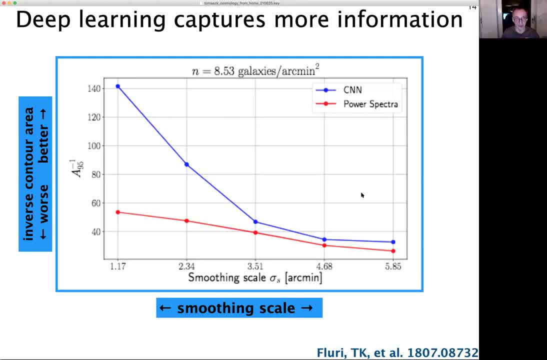 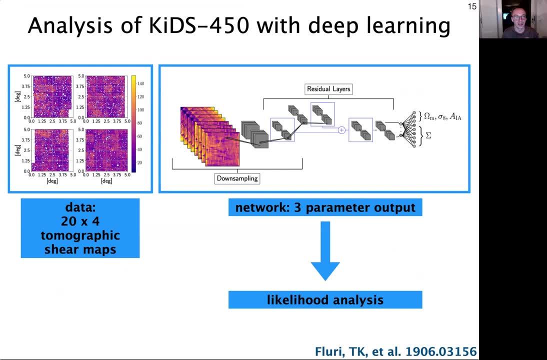 really, really significant over power spectrum that has access to the same scales um. so, equipped with this promising forecast, we proceeded to making the first kits, uh, the first measurement of cosmology parameters from kits. for fairest, for the future one, we stopped utilizing the fritillas Somerset Magnetic jersey on the top right and put on some CR灭s. If you have any questions, feel free to lot to ask or write on a form below. in the description, Just wanting to hear rank data, the evidence was in at the bottom of this video, so it's important to feel free to assezper. scroll to the forth. 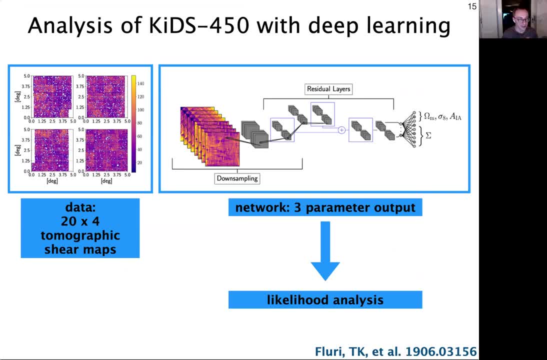 What if we try to implement our own ideas? Wewriter's work is going to go into a�� program over the fall 50 data with deep learning And this was a tomographic set up this time And we used a relatively deep residual neural net. 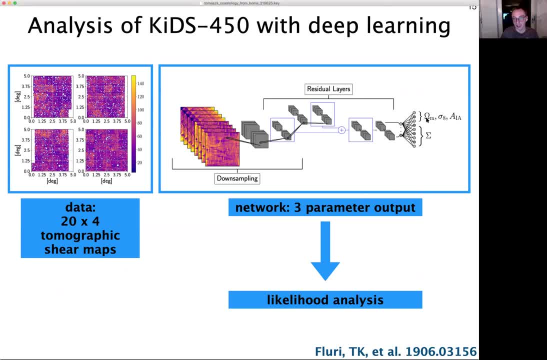 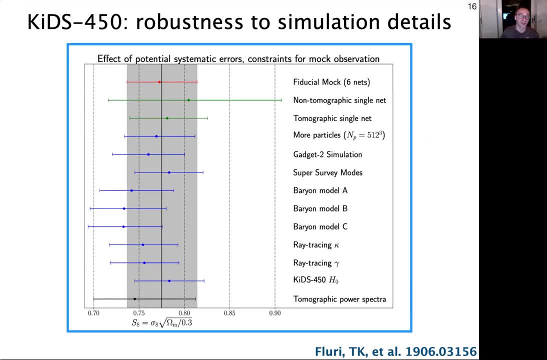 and predicted the parameters for omega M, sigma eight and intrinsic alignment amplitude. There was a blinded analysis, So the we did not look at the results until we were completely sure that our simulation and analysis methods are robust. So we tested a number of scenarios. 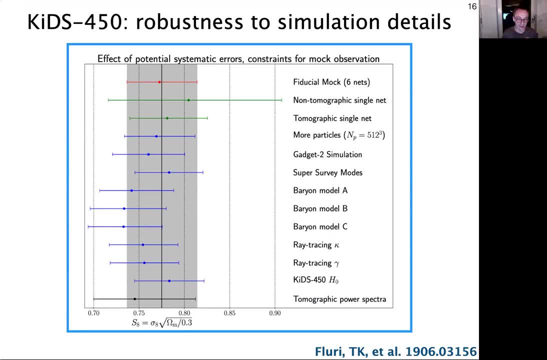 where we varied simulation parameters just to check if networks are robust to that, And most of the pretty much all the standard parameters in simulations don't play a role. So deep learning's robust learning in learning features that are actually physical rather than specific to a given simulation setup. 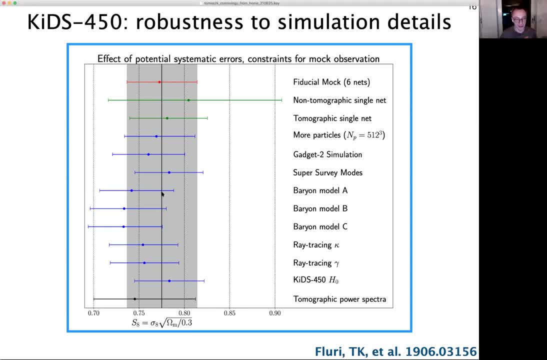 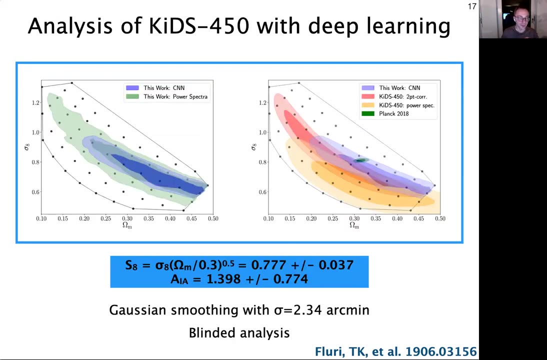 Of course we found that baryon models have very significant impact On kind of one borderline for this measurement. but for the future we'll have definitely a significant impact. So this was a limitation in the analysis. So with that we unblinded the results. 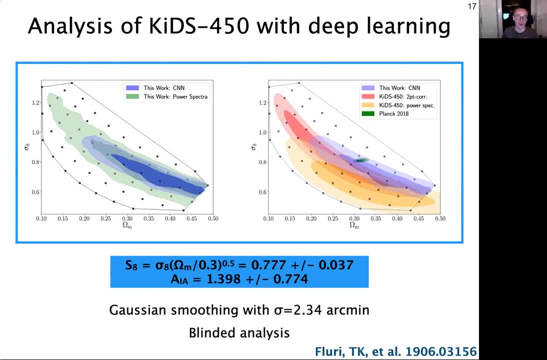 and we found that a new constraints on kids: 450 data using deep learning. We also compared it to our own power spectrum analysis in a apples to apples way again. So, as we expected, on the left side we see that CNN based measurement is smaller. 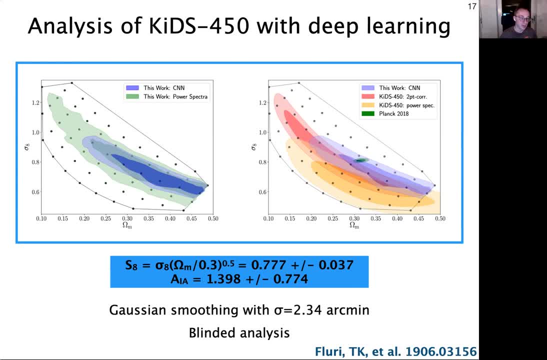 than the amount we achieved with power spectrum by the amount we expected it to have- around 40%- And also shrunk the degeneracy direction a little bit in the S8 Omega M banana shape, And we also found that we compared to other measurements. 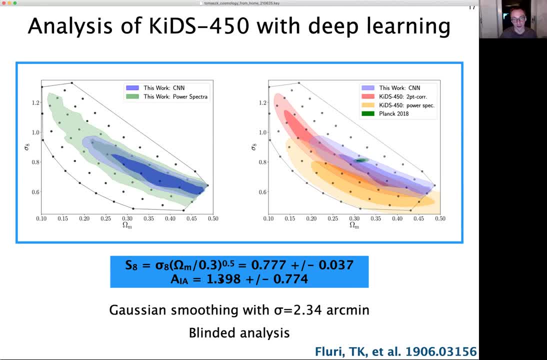 we found slightly higher Sigma eight and slightly higher intrinsic alignment amplitude. So we found that it was a little bit higher than that. So our measurement puts Sigma eight slightly higher than the main kids 450 measurement. So that's a very promising result And with that in mind, 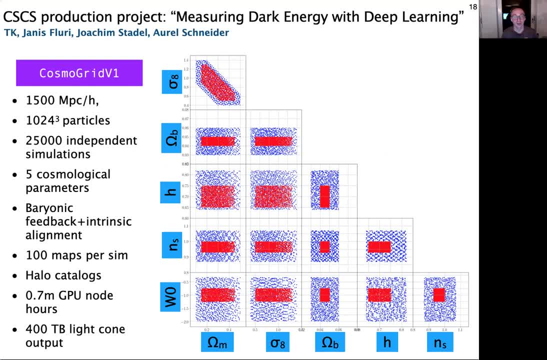 we proceeded to thinking about the future And of course, we will need a much improved simulation grid. So building a theory, a fully numerical theory prediction for Lambda CDM will be necessary for this deep learning methods to be applied. So we will need a much improved simulation grid. So building a theory, a fully numerical theory prediction for Lambda CDM will be necessary for this deep learning methods to be applied. 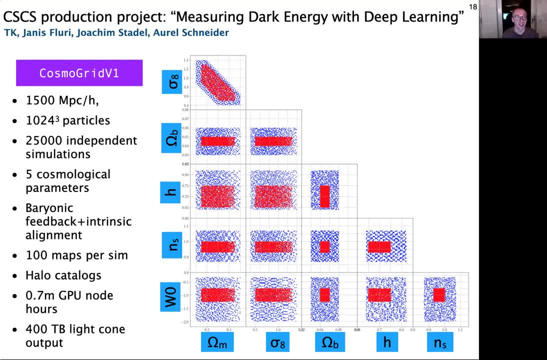 So we will need a much improved simulation grid. So building a theory, a fully numerical theory prediction for Lambda CDM will be necessary for this deep learning methods to be applied. So I led the CSCS production project called measuring dark energy with deep learning. 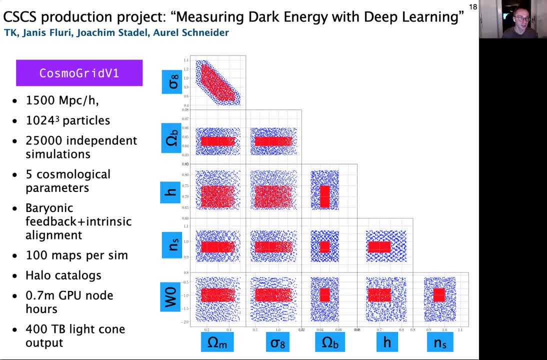 which is a collaboration between ETH, Zurich, University of Zurich and the Swiss Supercomputing Center. So this data is going to be finalized and we use it for putting deep learning based constraints in future lensing data. Also, what we will need is to work on the sphere. 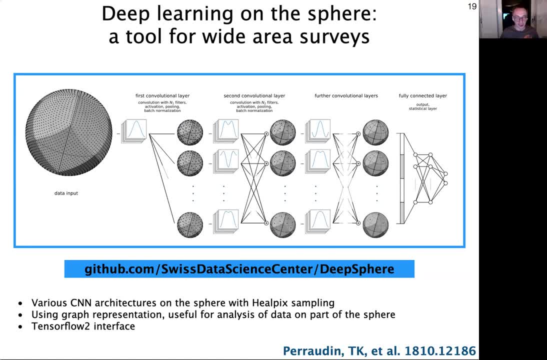 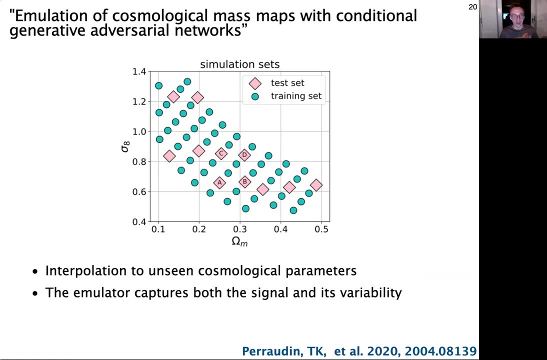 given that survey area is becoming large. So we developed this convolution neural network framework. So we developed this convolution neural network framework that is a public code that encodes a Hilpix pixelization and allows to build deep learning models. And second part of the talk. 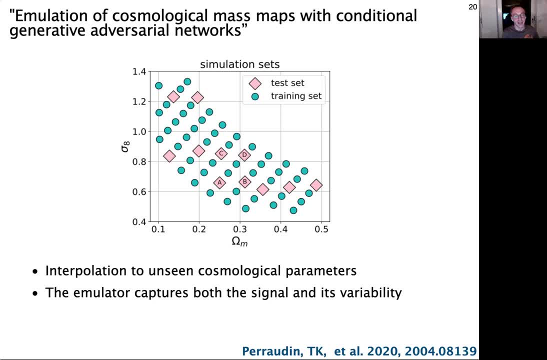 I would like to talk about using AI to generate simulations. I would like to talk about using AI to generate simulations for cosmological applications. So even now, for measurements based on power, spectra, we heavily rely on and body simulations calibration: we heavily rely on, and body simulations calibration. 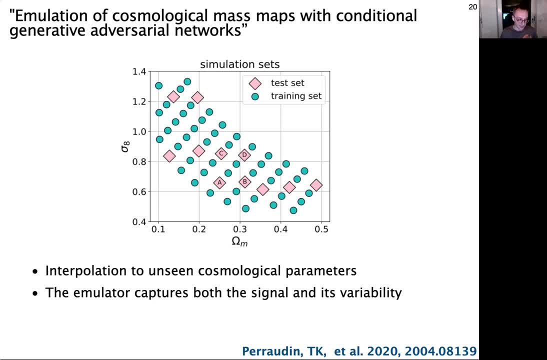 so for the non-linear part, and this is thetycznie done by creating emulators of the P OF K. examples are, for example, Euclid emulator, Cosmic, MU or Bucko, And they're very fast and very precise emulators built on and body data. 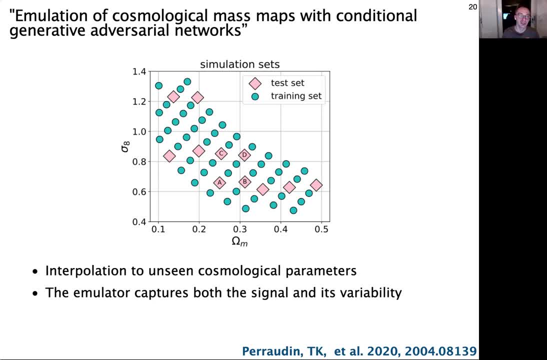 So to reach needed precision levels. we need to use simulations whenever we do so to reach the needed precision levels. whatever we do, whatever we- whether it's power spectrum based analysis or deep learning analysis of building emulators- we thought: why not try to build an emulator for the mass maps themselves? 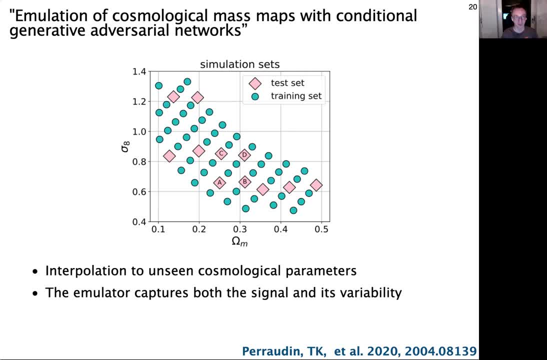 for a given survey scenario. So we worked on this for in a series of papers, but in the latest paper we published, we used conditional generative adversarial networks, which is a type of generative AI which we trained on a grid of simulations from here in this picture: 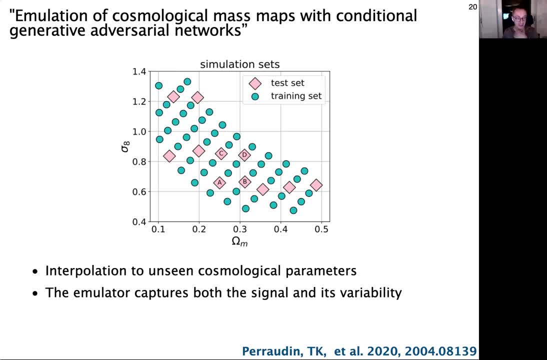 and it was done in a conditional way so that we can ask- once the generator is trained, we can ask it for to give us a an example mass map at any point inside the grid so it can interpolate between the points in terms of inside the generative model and, most more importantly, 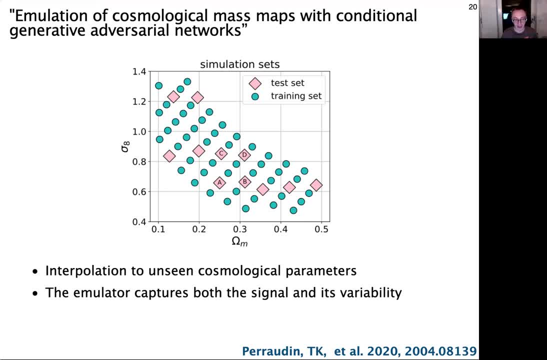 this emulator captures both the signal, so the how the mass looks like, and its variability, so how the mass differs if we use different random seeds but keep the cosmology fixed. So we tested both the aspect of how accurate it we are modeling its signal and the variability using generative adversarial nets. and 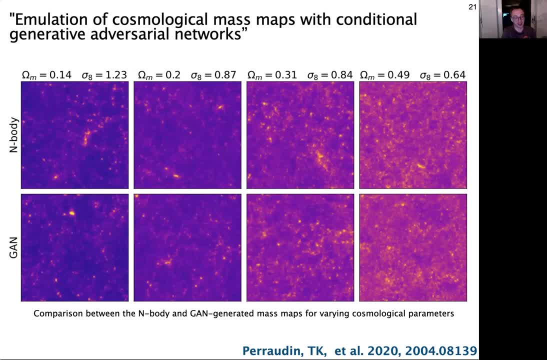 performed a very extensive series of tests. of course, we started with a visual comparison, and for different cosmologies- GAN and NBody- images of mass maps look practically indistinguishable. note that these four cosmologies are chosen so to be at different parts of this parameter space. 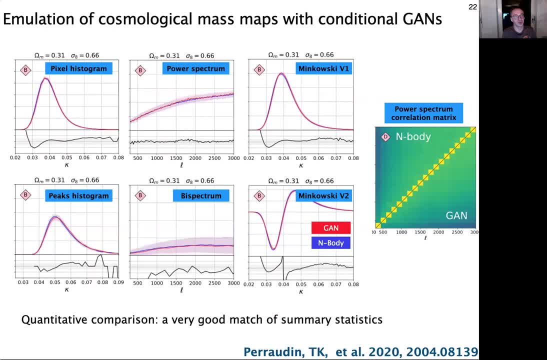 you can clearly see the difference by eye and also perform quantitative analysis, which was done using standard summary statistics, using cosmology power spectra by spectra Minkowski functionals and also, importantly, we compared covariance matrices of power spectra that come from. a sample of maps were generated with NBody and with GANs. these points shown here: 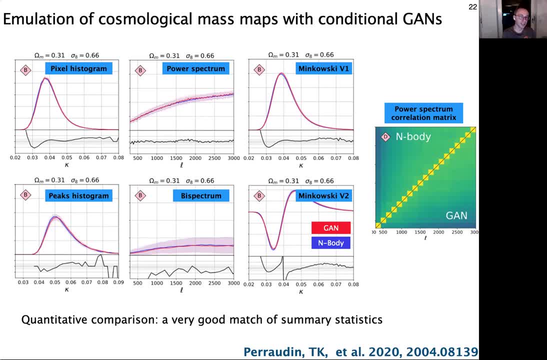 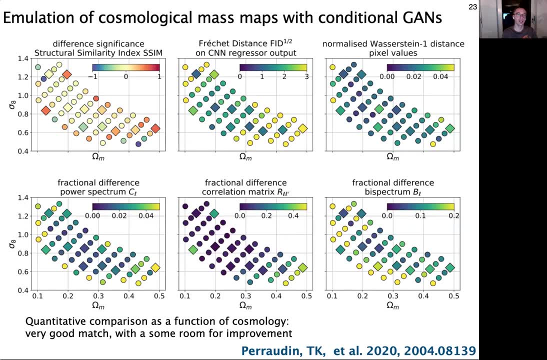 are for cosmologies that were not included in the training set, so this is testing the ability of the network to interpolate in this data space. finally, this is a comparison of how stable these results are across the entire cosmology grid, and we used all sorts of different metrics to compare. the metrics on the in the bottom row show the typical. 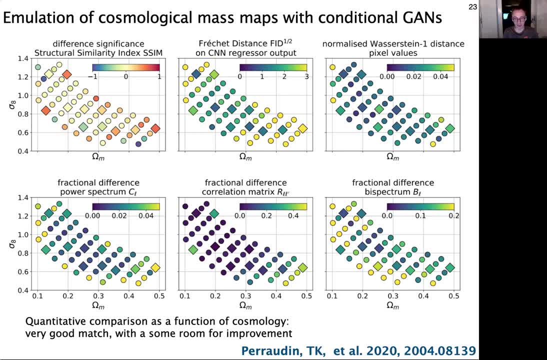 cosmological summary statistics: power spectra, correlation matrix and bispectra. and the top show, the one sigma shift will have a value of one on this color bar, for if everything was a gaussian distribution? so it gives a little bit of intuition about the scale of the problem here, and we mostly 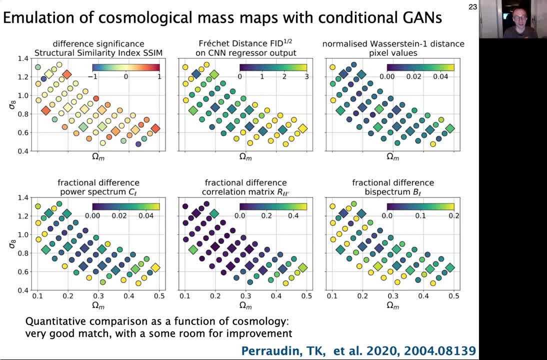 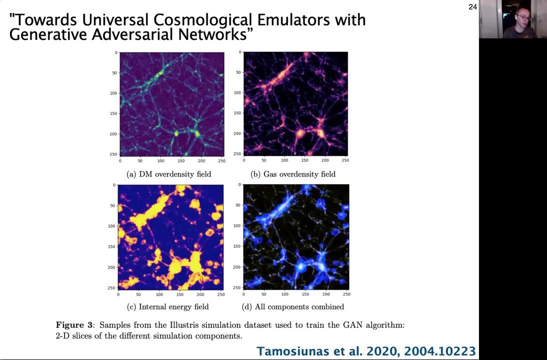 can match all of these quality metrics to a couple of percent across the entire simulation grid, with an exception maybe of a bispectrum which has some regions where it's matching a bit worse and some extremes there in the structural similarity in the directs as well. so generative adversarial nets we demonstrated as a tool for generating. 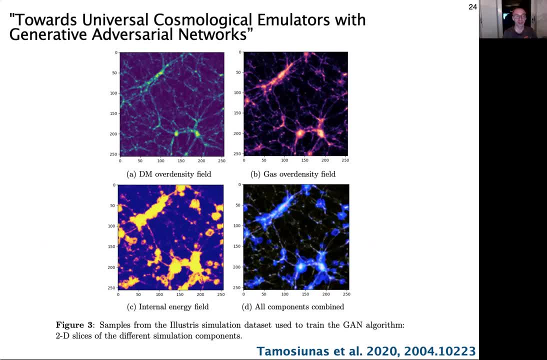 density or maps of density fields, and there was also quite a lot of work on simultaneously generating different types of observables in one go. for example, in this excellent work by the team in portsmouth, guns were demonstrated to be able to predict multiple observers at a time such as dark. 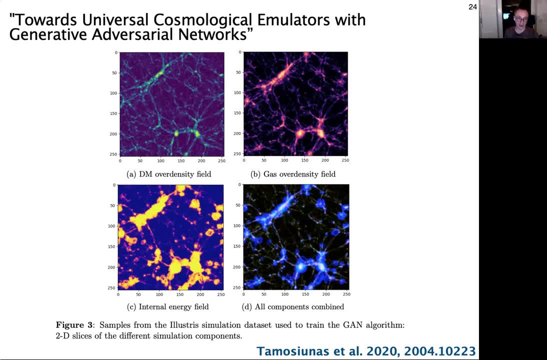 matter of a density field and gas field, internal energy field, and so this can be also potentially used to to uh uh in paint barion feedback models onto dark matter simulations and basically um test uh, the enable also small scale inference um using simulations and deep learning methods. 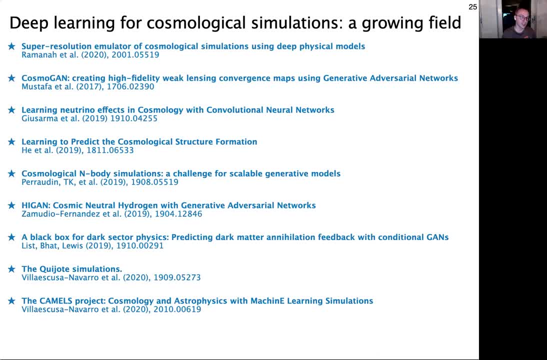 um, this is a growing field, so i've been a number of papers demonstrating how cosmological simulations can be helped with use of deep learning or ai, and- and I think this is going to be playing a more important role in the future due to this fantastic ability of AI to generate non-linear models. 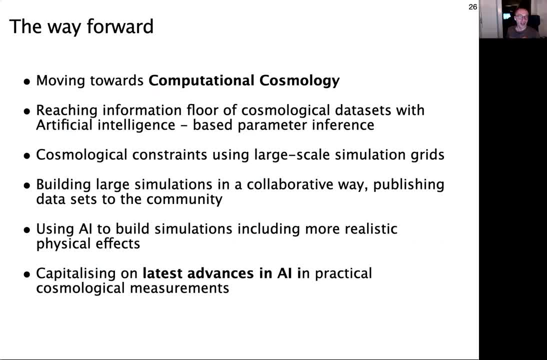 This is the end of my talk. Thank you very much for your attention. Just to point towards several ways to go forward with machine learning in cosmology. I think we are moving towards the computational cosmology where more and more aspects of the analysis are done numerically and with that we can actually try to reach 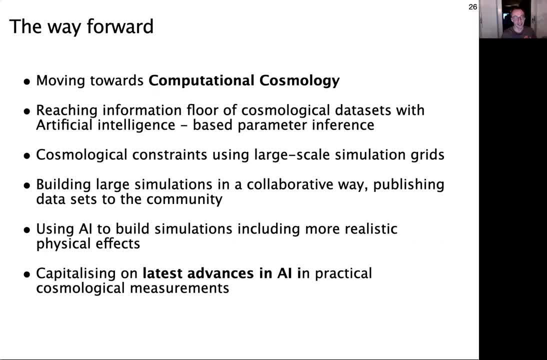 the information floor of cosmological data sets using AI. This is due to their feature of automated pattern extraction and using this AI tools for cosmological inference. We will use large-scale simulation grids. The construction of these grids is computationally very expensive, so I think large collaborative efforts will be. 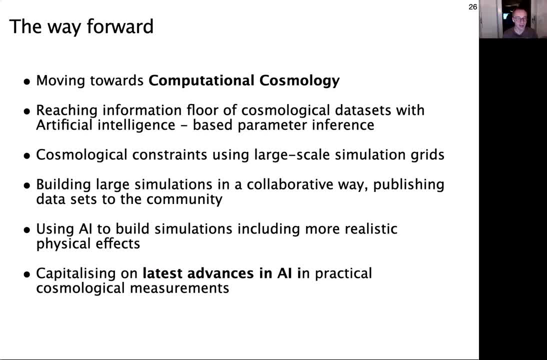 quite important here, especially publishing data to the community. Together with building the simulations, we can try to understand our astrophysical effects in simulations better. For example, baryonic feedback or other types of effects can be really useful for modeling, simulations and AI. 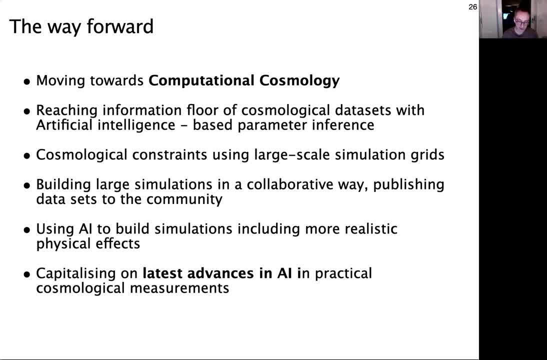 Finally, one last thought is that the advances in AI will continue to accelerate due to the powerful applications in the industry. A lot of these tools are being made public to the community, especially for scientists, so I think we can capitalize on this progress and reap this long-hanging fruit of. 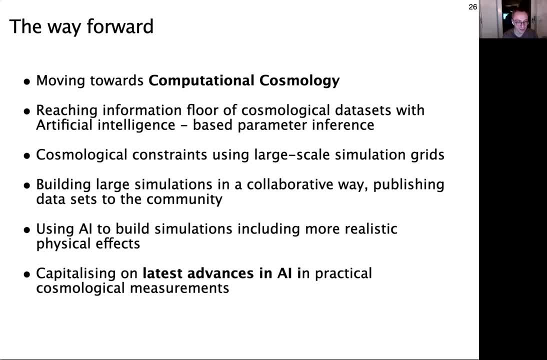 using AI for increasing our precision of cosmological measurements. Thank you very much.